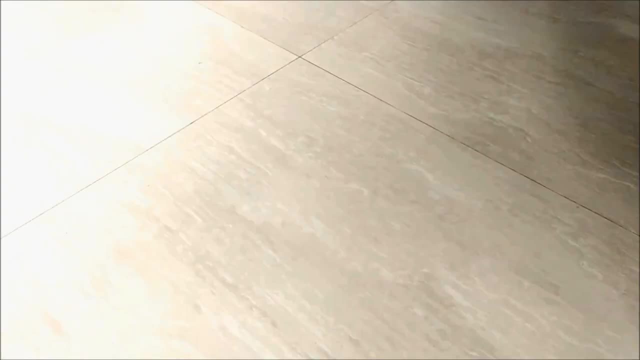 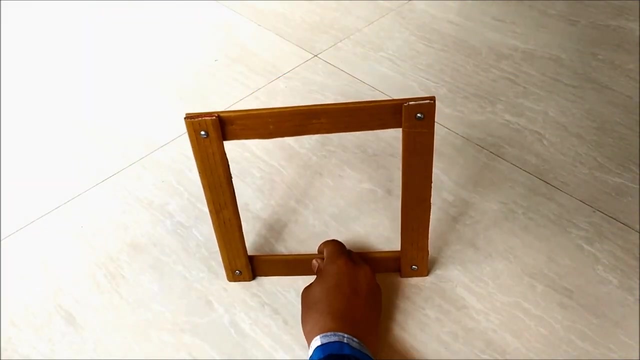 their proportions and maintains its saving position. If you make a square from four pieces of cardboard with built connection at their joints so that all members can free to rotate When force is applied, you will find that it doesn't stay square. It can easily be transformed. 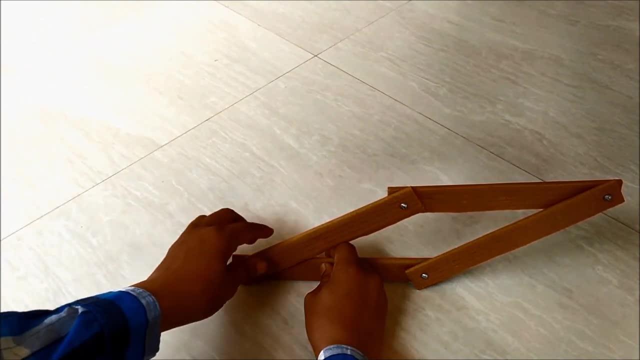 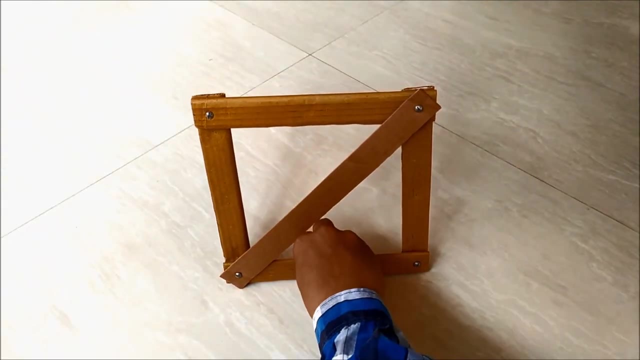 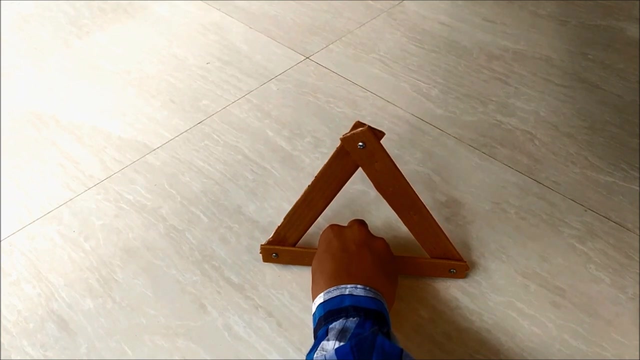 into a parallelogram and collapse when subjected to a little force. Now if you place one diagonal piece from corner to corner, doing that makes two triangles. Now this is more strong and stable. Or if you make a triangle from three pieces of cardboard with pinned connection at their. 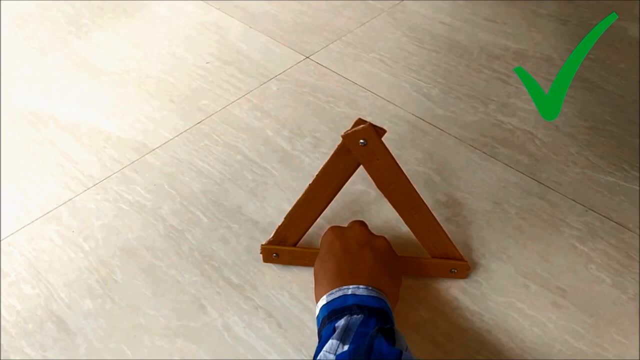 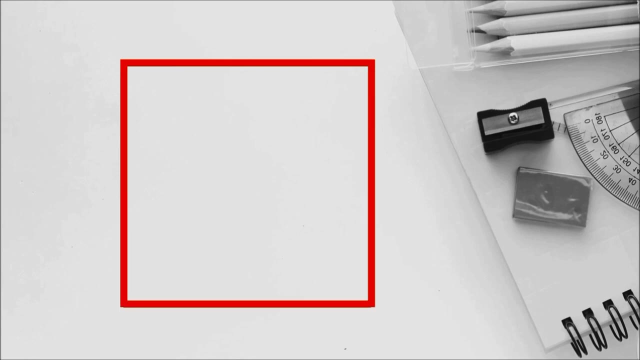 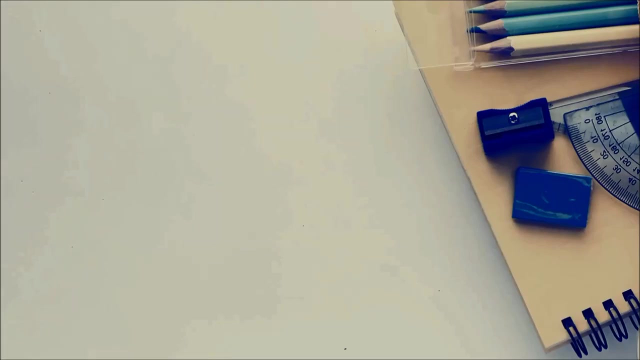 joints. When force is applied, you will find that this is more stable and stronger than the square. The reason behind this scenario is squares are made up of four sides, But you can change the angles to get any quadrilateral shape with that same sides, But triangles. 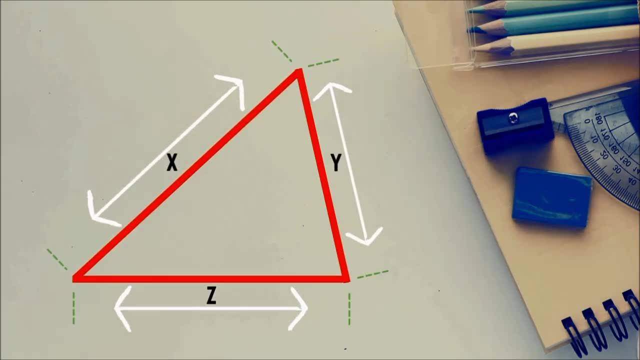 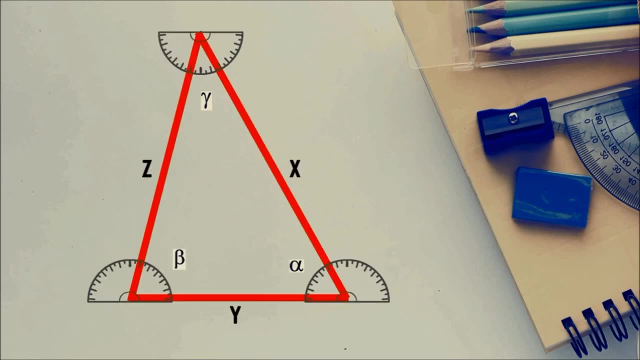 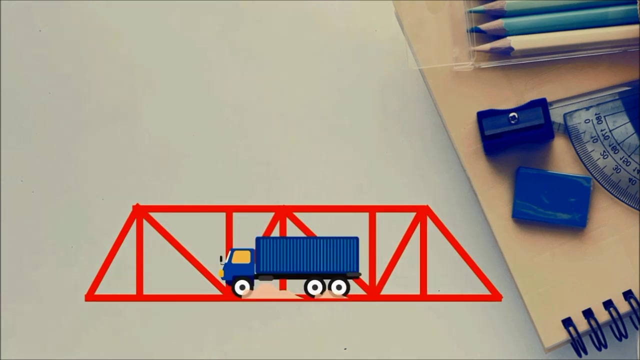 are different, having three sides with valid length and you can't change the angles to a new triangle with that same sides, as there is exactly one triangle that you can make from those sides. this is how triangles hold their shape and, by interconnecting, carry relatively heavy loads in. 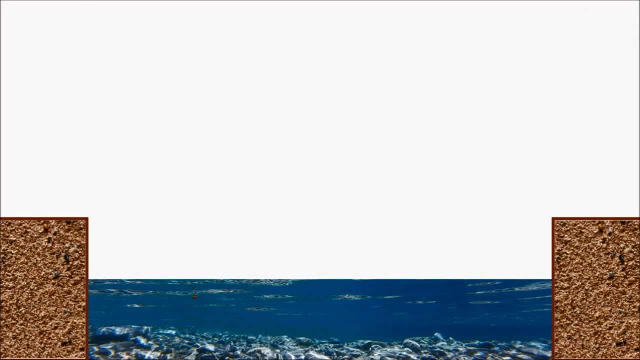 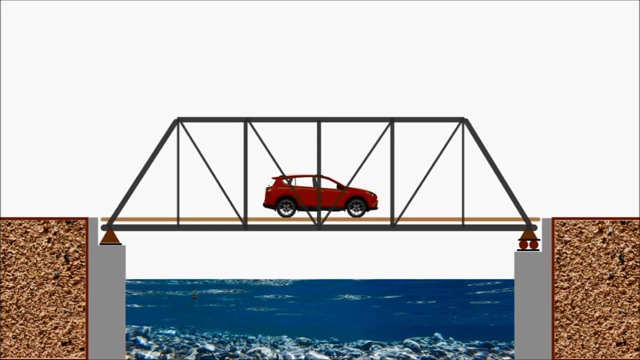 truss bridges. a truss beach mainly consists of abutment which supports the end of the superstructure, bearing and pedestals which transfers the superstructure, loads and movements to the substructure: bottom chord, top chord end, post, vertical, hip, vertical diagonal and deck slab. a single span, truss, which is like a simply supported beam because it carries vertical. 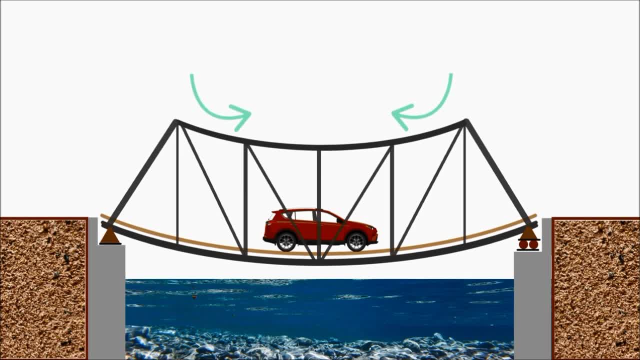 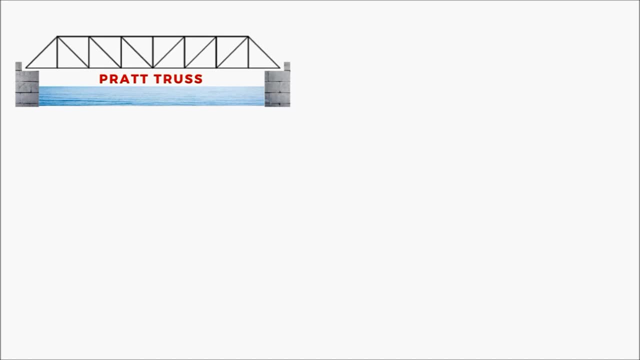 loads by bending. bending leads to compression in the top chord, tension in the bottom chord and either tension or compression in the vertical and diagonal members, depending on their orientation, and according to this orientation, over 30 different types of truss bridges are out there, in which some basic types of truss bridges we will discuss today, which are most commonly used. 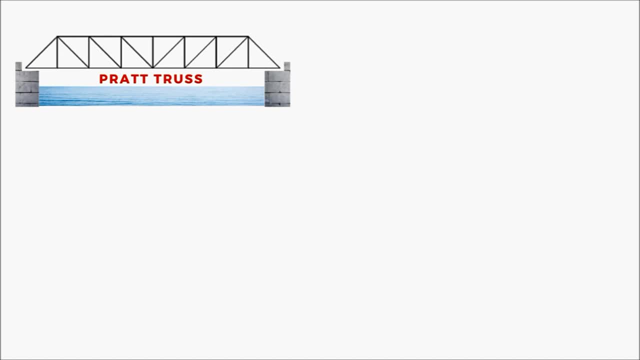 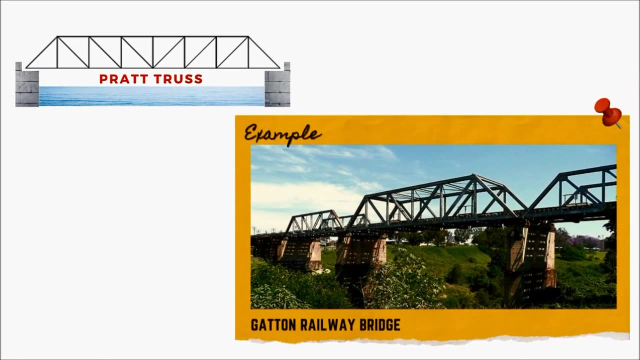 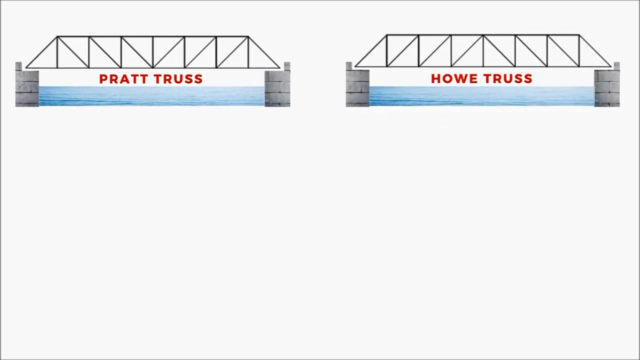 prac truss includes vertical members and diagonals. each diagonal member slopes in downward direction toward the middle of the beach. gurton railway beach in australia is an example of prac truss b, the howe truss bridge, which, opposite of the presumably design, where each diagonal member slopes in the upward direction toward the 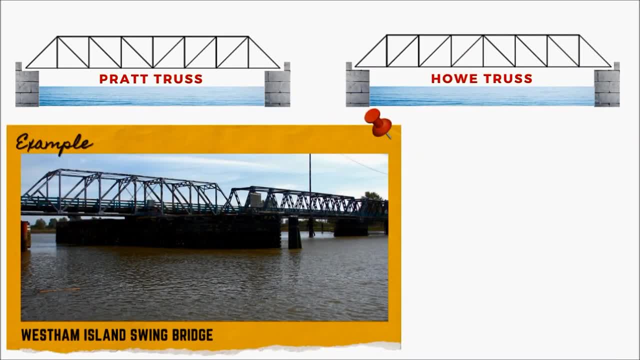 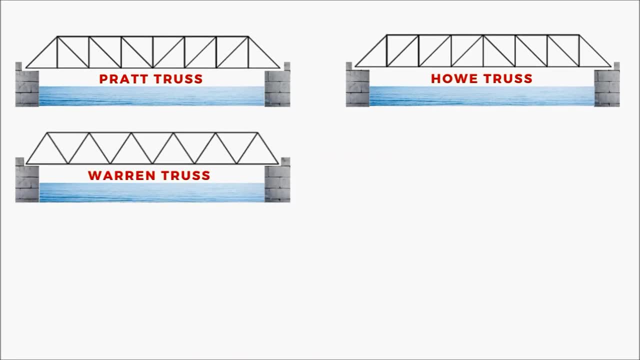 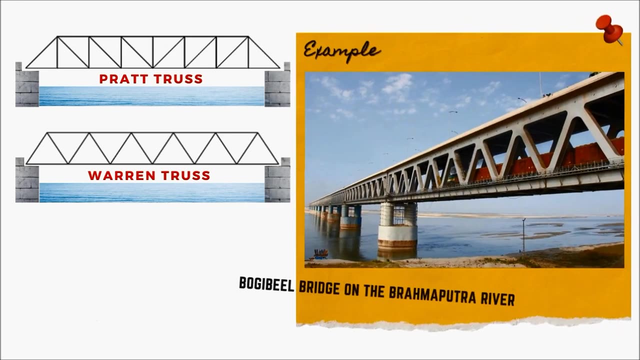 middle of the bridge. Western Island Swing Bridge in Columbia is an example of Howe Truss Bridge. Warren Truss includes only diagonal members. No vertical members are there. It consists of placing equilateral triangles along its length. Boggyville Bridge and Brahmaputra River in Assam is a great 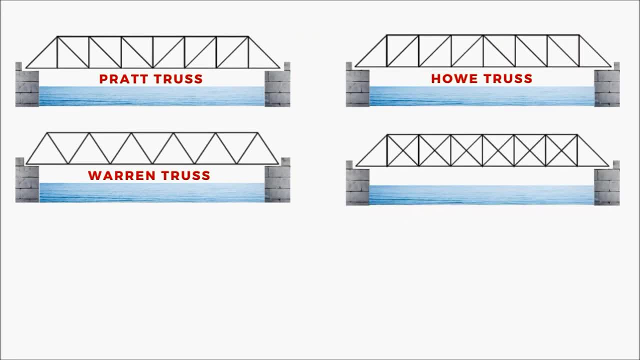 example of Warren Truss Bridge. Brown Truss is the combination of Bragg Truss and Howe Truss, where diagonal members slope in the downward and upward direction toward the middle of the bridge. White's Bridge in United States is an example of Brown Truss Bridge. The K Truss is named after K, formed back to. 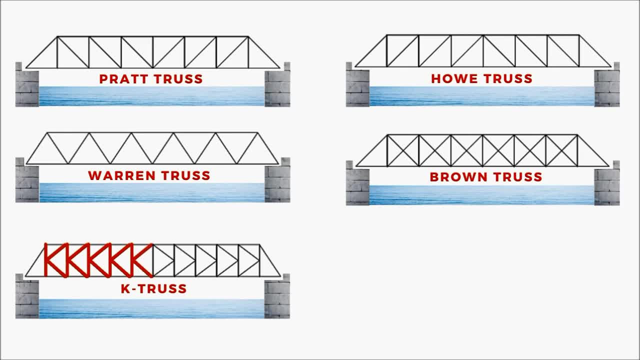 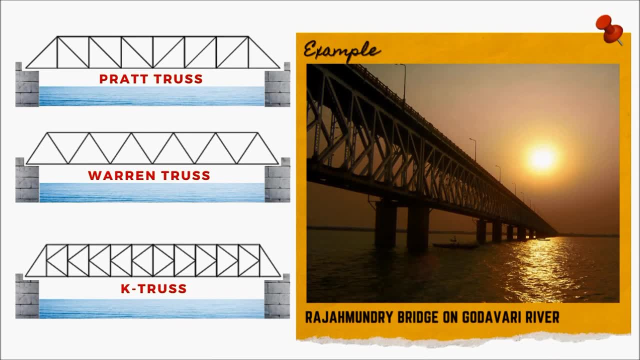 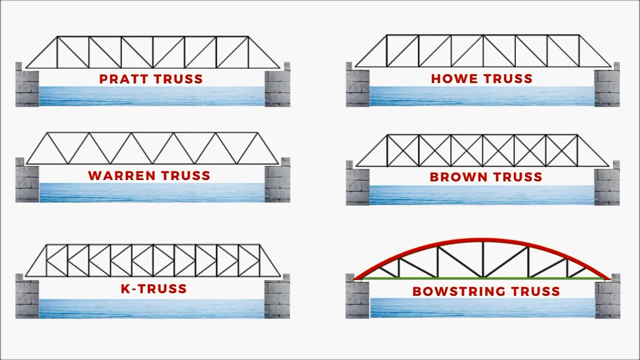 back in each panel by vertical members and two oblique members. Rajahmundry Bridge on Godavari River in Andhra Pradesh is an example of K Truss Bridge. The Bow String Truss consists of an arch top chord with vertical and diagonal members running along the span of the bridge. The 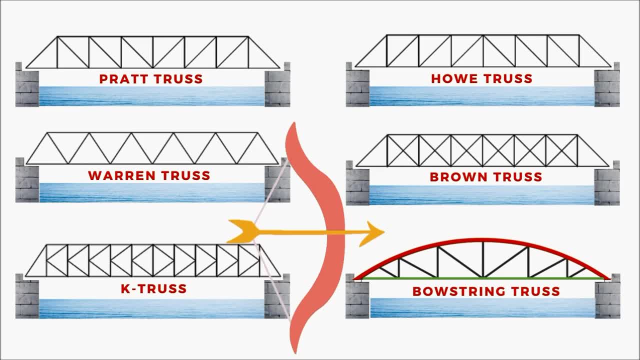 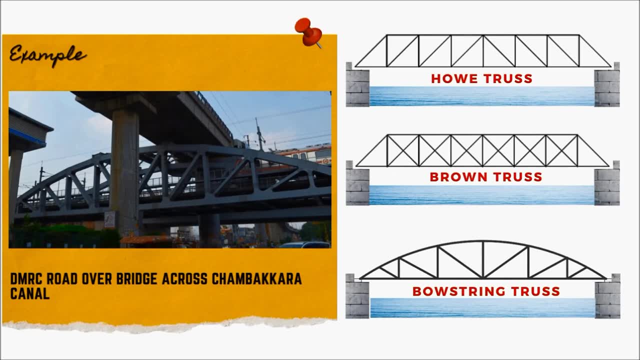 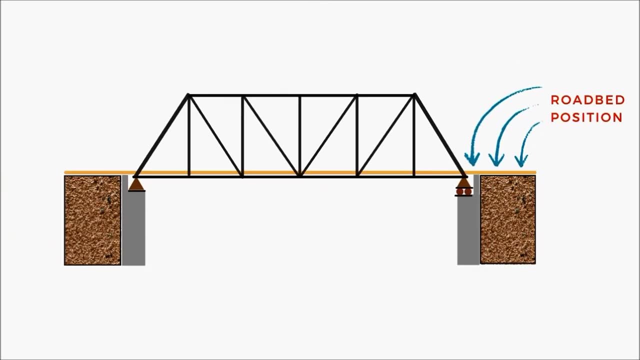 arch tied with bottom chord looks similar to bow string, Hence the name formed. DMRC. Road Over Bridge across Chamvakra Canal in New Delhi is an example of Bow String Truss Bridge And the truss bridges can be classified in three types, according to the roadbed position. 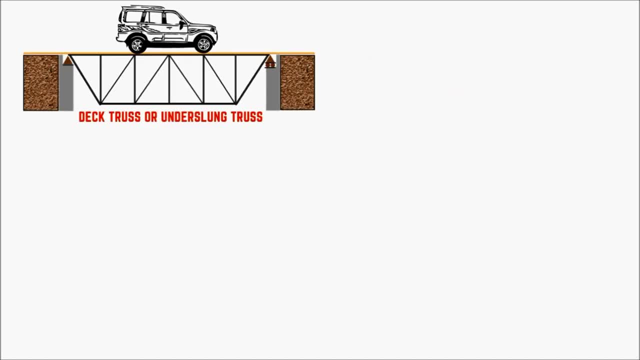 When the roadbed is in the top of the truss, it's called a deck truss or underslung truss. If you look at the cross section of the truss, you can see that both sides are connected and forming box shape. When the roadbed is in the middle or bottom of the 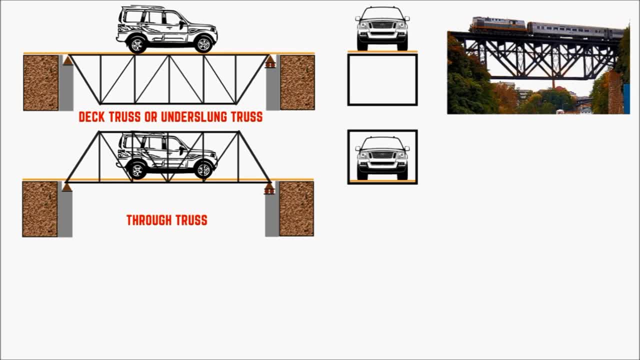 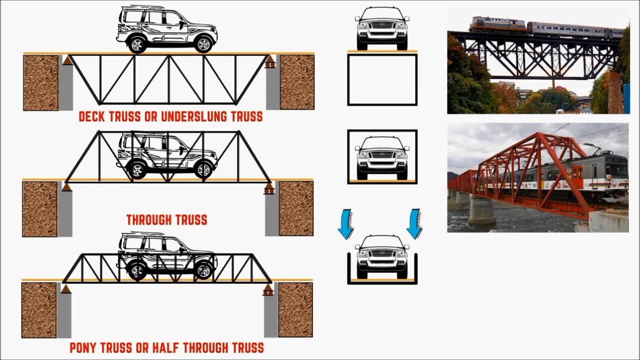 truss, it's called a through truss And here also the truss in both sides are connected and forming box shape. And when the roadbed is in the middle and bottom of the low height truss which are not connected with each other, it's called as a pony truss or half through. 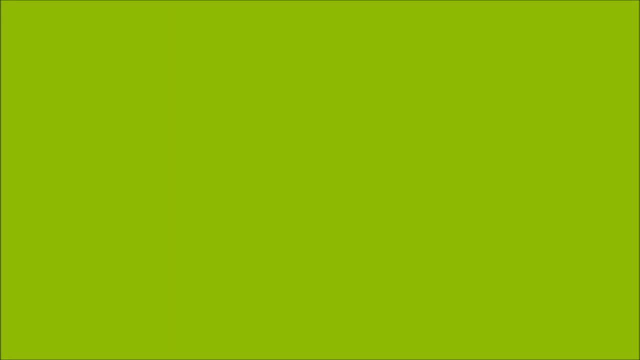 truss. There are some assumptions made for the analysis of simple truss. 1. all members in truss are connected together by frictionless pin connection so that all members can free to rotate at joints. 2. truss members are connected together at their ends only, which means loads are only. 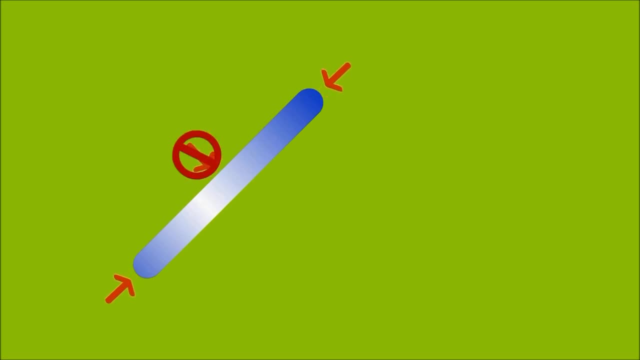 ever applied at their joints of the truss. no loads to be there in the middle of any members. 3., 3. 3. bending moments. because all joints are pinned, They can only carry axial force. Each member has to be in equilibrium, So the forces acting at each end of the member must be equal and 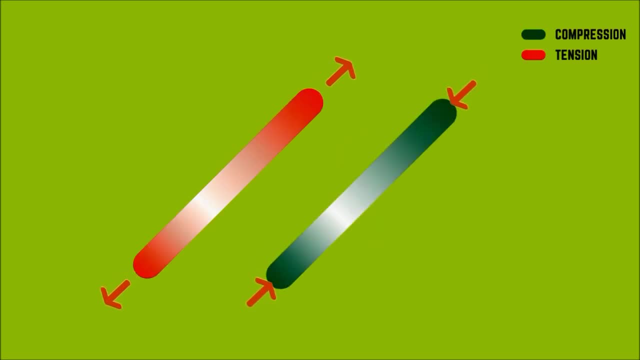 opposite. Each and every member is either in tension or in compression. Now, to determine which members are under tension and which members are in compression, we need to analyze the truss. There are two methods for analysis of a simple truss. Method of: 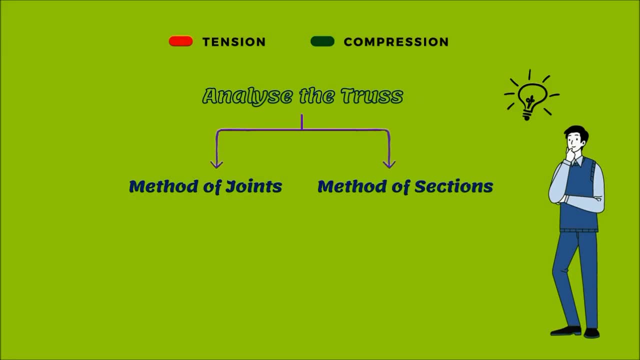 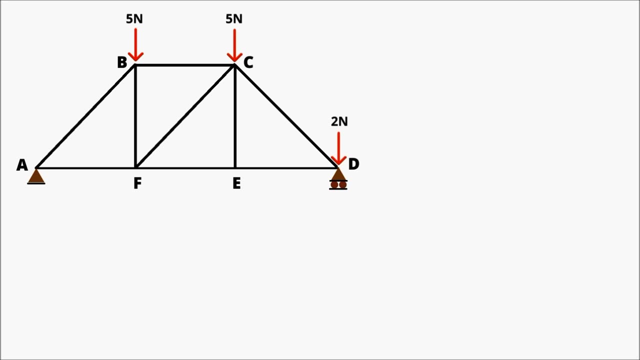 joints and method of sections. In this video we will analyze the truss by method of joints. This is a simple truss with some external loads And there are three steps in method of joints. Number one: we need to know the equations of equilibrium. Number two: draw. 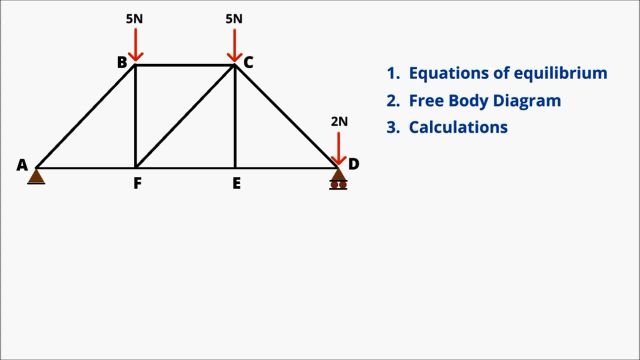 the free body diagram And number three calculations. There are three equations of equilibrium in a 2D space: 1. Position of all the forces in X direction will be zero. 2. Summation of all the forces in Y direction will be zero and. 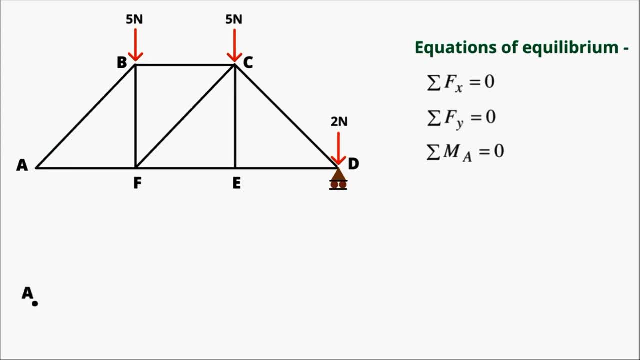 3. Summation of all the movements: each equals to zero. Now at point A there's a pin joint, you can see. So we will have X and Y reaction at point A and roller at point B. So we only have a wide reaction at point D. There are some. 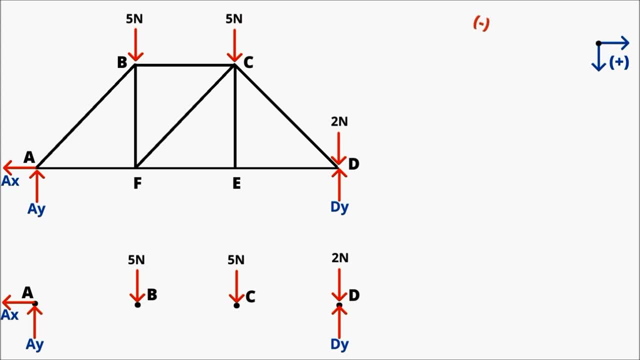 forces acting rightward and downward as positive and leftward and upward as negative. You can assume the opposite of it. By summing the forces in x direction, we get minus ax equals to 0 or ax equals to 0. So we are erasing ax from the diagram Now by summing the moments about point. 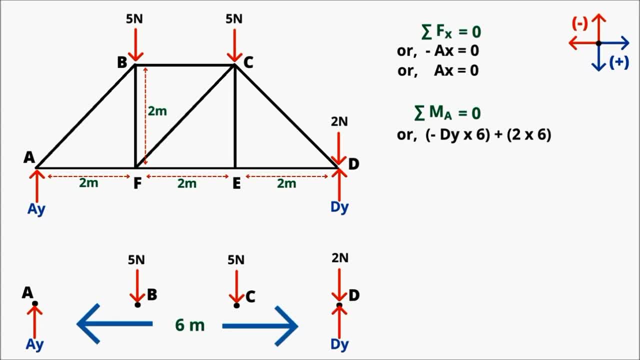 a. we get minus dy into 6 plus 2, into 6 plus 5, into 4 plus 5 into 2 equals to 0, or dy equals to 7 newton. So we are replacing dy at 7 newton in the diagram. Now summing the forces in y direction. 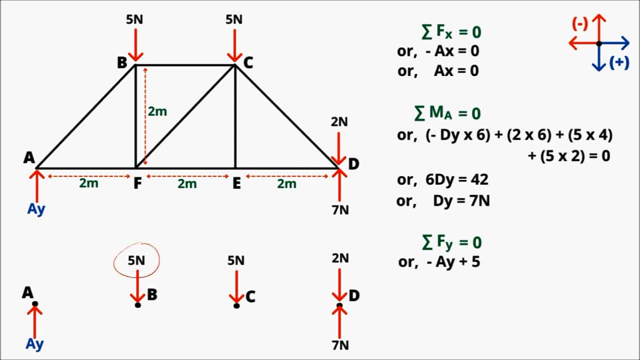 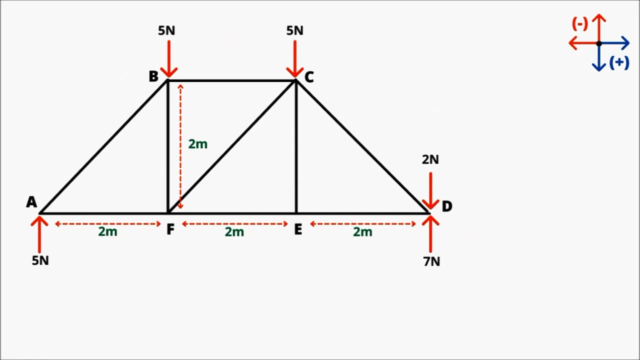 we get minus ay plus 5 plus 5 plus 2 minus 7 equals to 0, or ay equals to 5 newton. So we are replacing ay as 5 newton. Now step 2.. Let us draw the free body diagram. 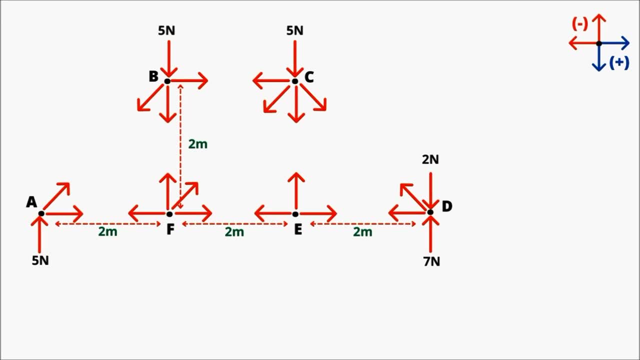 It's nothing but showing the forces through the members from the joints itself. You can assume all the members of the truss are either in tension or in compression. Here we are assuming that all members are in tension- Wait what I said- tension. But the force are showing inward direction to the 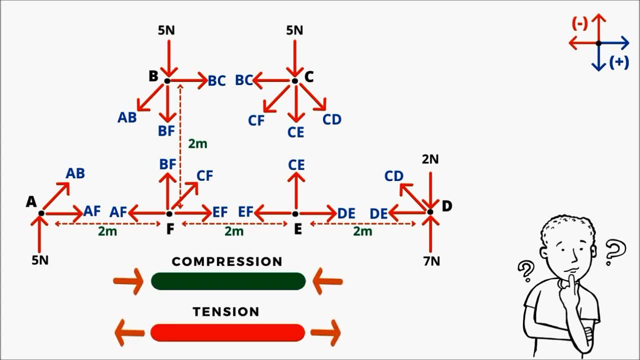 members in the diagram And we know the force acting outward is equal to the force acting outward. So we are replacing ay as 5 newton. Now step 2.. Let us draw the free body diagram. It's nothing but showing the forces through the members. from the joints itself You can assume all the 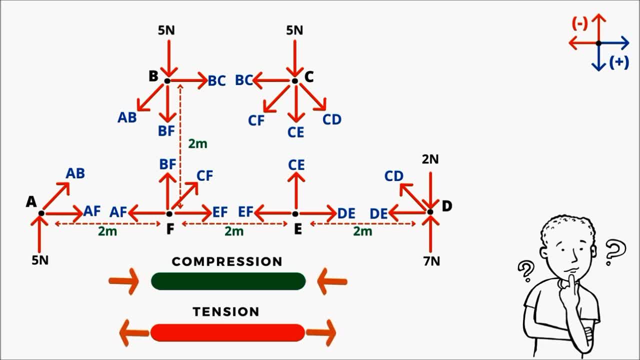 members of the truss are either in tension or in compression. Here we are assuming all the members of the truss are either in tension or in compression And we know the force acting outward direction is called as a tensile force, which pulls the members right Here most of the 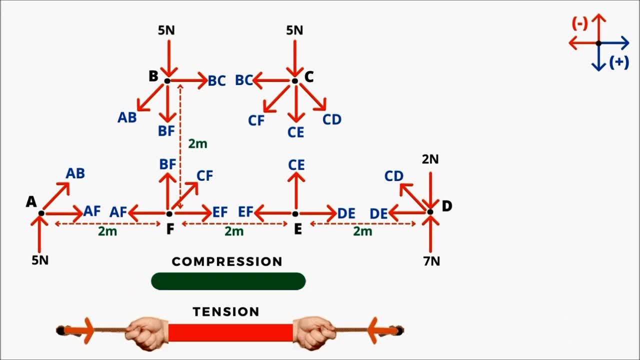 students get confused. When we talk about the member being under tension, it actually pulls the joints to elongate itself. It's nothing but the Newton's third law of motion. For every action there is an equal and opposite reaction. And when we talk about the member being under compression, 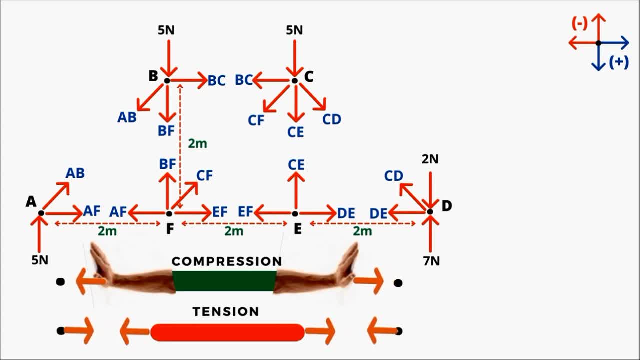 it actually pulls the joints to squeeze itself. So in method of joints, when we draw the free body diagram, the force in outward direction is compression and inward direction is tension. now we are assuming all members are in tension if after calculations we get negative value for 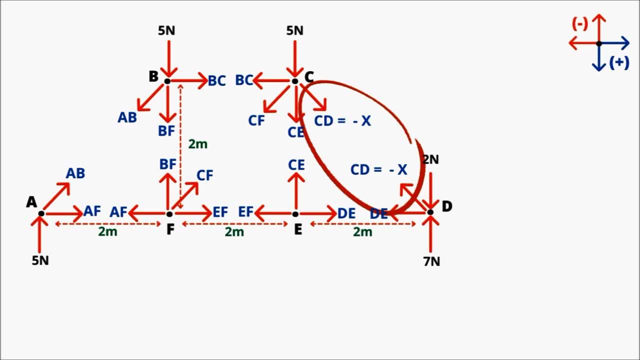 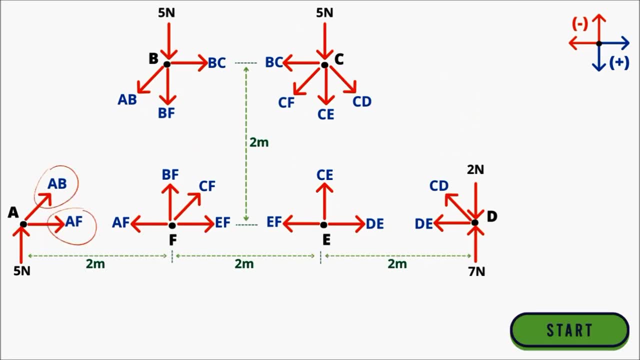 any member. that means we guessed wrong. that particular member is actually in compression. now to decide where to start the analysis, we need to find a joint where there are only two unknown forces. all members are pin jointed, so there are only two equilibrium equations and we can solve. 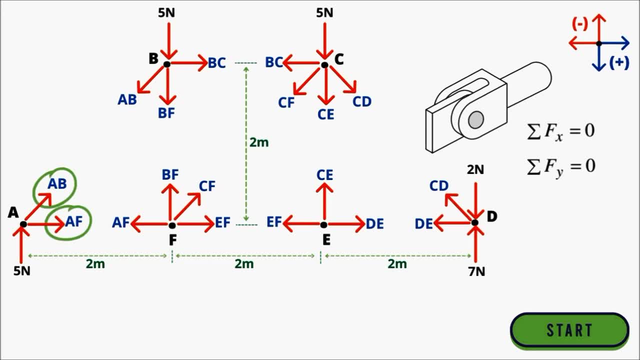 only two unknowns in this diagram, only point a and point b. both have two unknowns, so we can start from any of it. let's start the calculations from point a now. write the vertical and horizontal components of inclined member a- b by simple trigonometric formula, then apply the equilibrium. 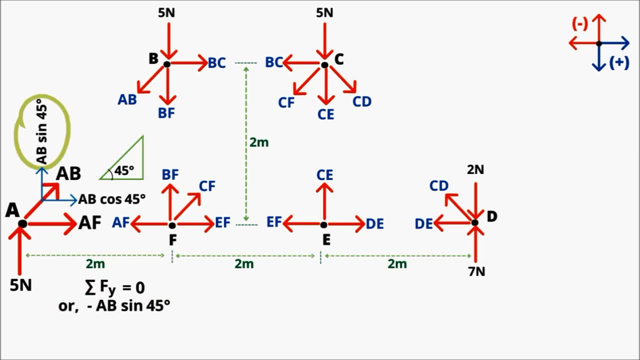 equations: summation of f? y equals to zero or minus a? v sine forty five minus five equals to zero. by simplifying this we get a? b equals to minus 5. root 2 newton means member a- b is in compression. now summation of f? x equals to 0 or a? b cos 45 plus a f equals. 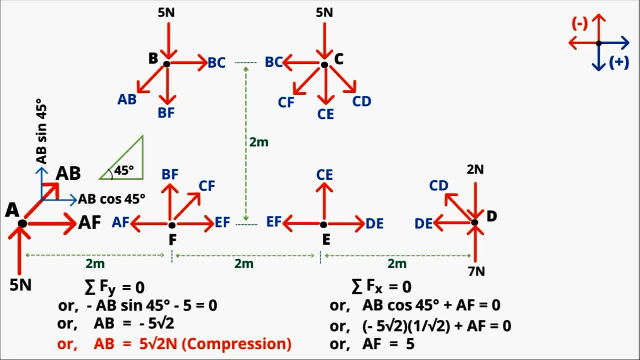 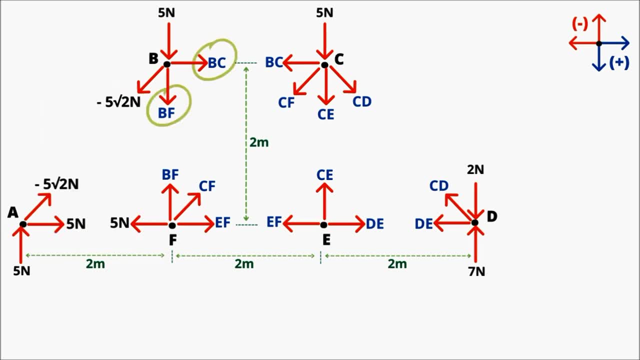 to 0. by simplifying this we get a f equals to 5. newton means member a f is in tension. now replace these values in the diagram. now point b has two unknowns. let's solve it by following same procedure. write the vertical and horizontal components. 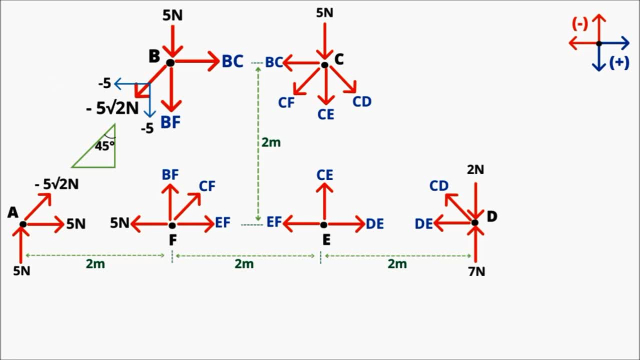 of a- b and simplify it. then apply the equilibrium equations: summation of f: y equals to 0 or 5 plus b. f plus minus 5 equals to 0 or b. f equals to 0 means member b. f is a. no force member now. 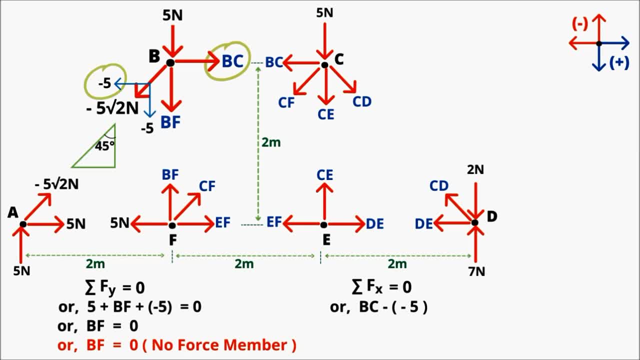 summation of f x equals to 0 or b c minus minus 5 equals to 0 or b c equals to minus 5. newton means member b c is in compression. now put these values in the diagram. now you can see point f has. 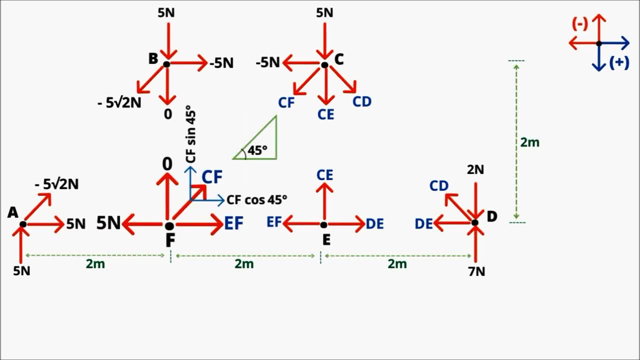 no force. in this equation, once again, follow the same procedure. write the vertical and horizontal component of inclined member, cf. summation of f. y equals to zero or minus c. f sine. forty five minus five equals to zero or c f equals to zero means c f is a no force member. now summation of. 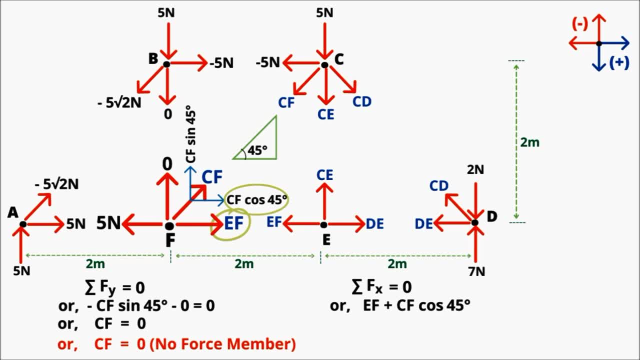 f x equals to zero or eu minus 5 equals to zero. em calculated by simplifying this, we get: ef equals to five. newton means number ef is in tension. pour these values in the diagram now. grind a哦-еу plus intention. Put these values in the diagram Now. point E has two unknowns. Summation of. 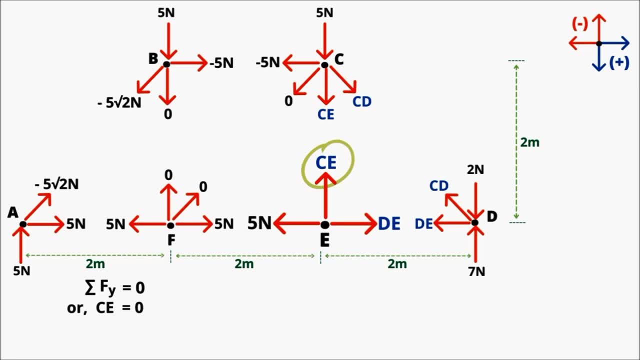 Fy equals to 0 or Ce equals to 0 means Ce is a no force member. Summation of Fx equals to 0 or De minus 5 equals to 0 or De equals to 5. newton means its intention. Now put these values in the. 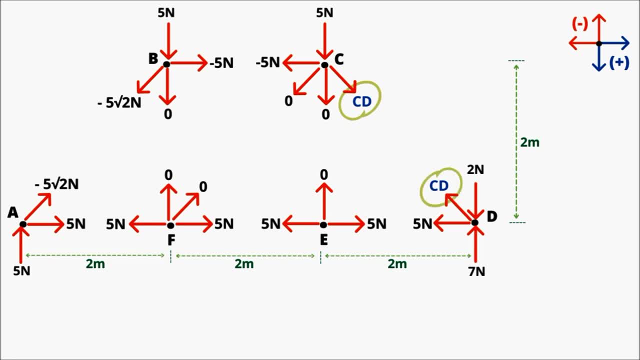 diagram. Now you can see point C and point D. both have one unknown. Let us solve point D. Write the vertical and horizontal components of CD. We need only one equilibrium equation to solve this. Summation of Fx equals to 0 or minus CD, cos 45 minus 5 equals to 0 or CD equals to minus 5. 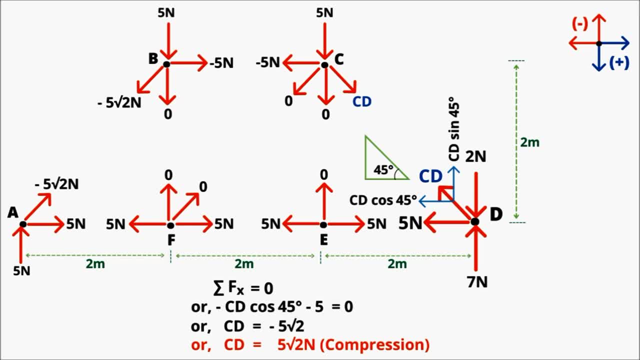 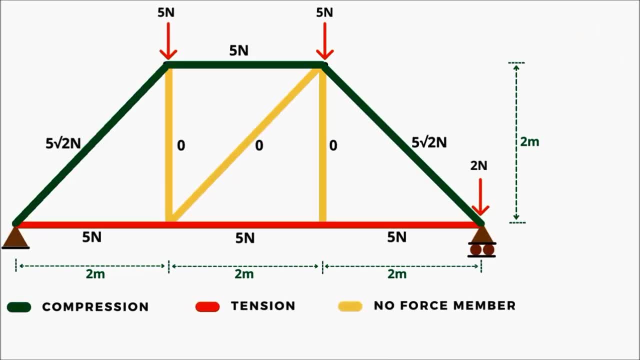 root 2. newton means its in compression. Finally, put the value in the diagram. We have completed the analysis of this simple truss. Now you can see which members are under tension and which members are in compression.